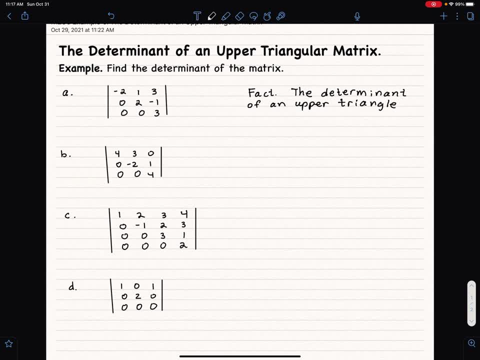 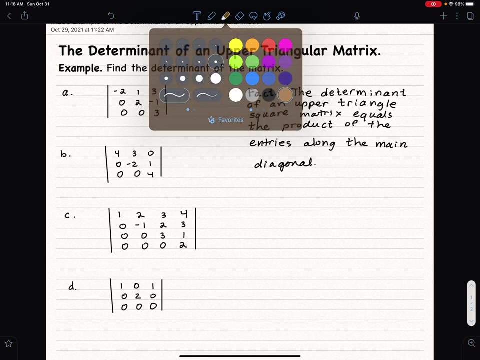 The matrix has to be square anyway for the determinant to make sense. but I'll say that Upper triangular square matrix equals the product of the terms of the entries. maybe entries is better entries along the main diagonal. Okay, well, in order to understand this, I guess what we need to do is even stop and think. 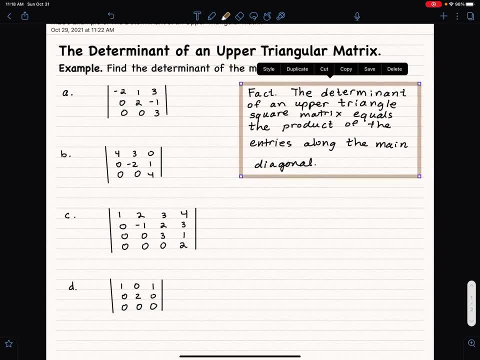 what does it mean? What does it mean for a tri-yaw matrix to be upper triangular? So what we have here is: and also, what's the main diagonal? Okay, let's start with the idea of a main diagonal. So the main diagonals are the ones that I'm is what I'm putting a thing around here. 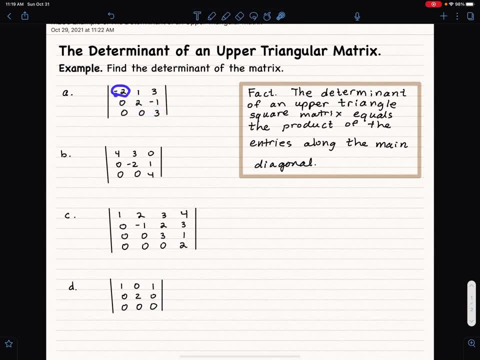 And it's those entries where the 1-1 entry, the 2-2 entry, the 3-3 entry, those are the main diagonals, Those where the row and column number are the same. So that's the main diagonal. 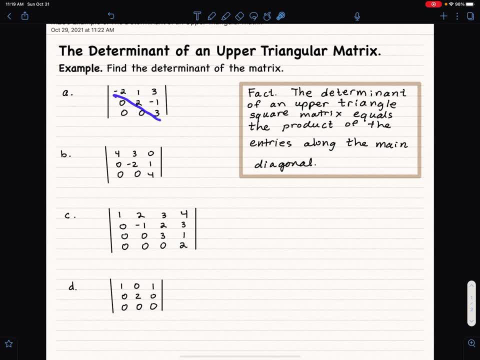 And upper triangular means that below all the entries below the main diagonal are zero. You could have entries zero above the main diagonal, like the second one here, But below the main diagonal we need all zeros. Okay, And so this guy here. this first one is in upper triangular form. 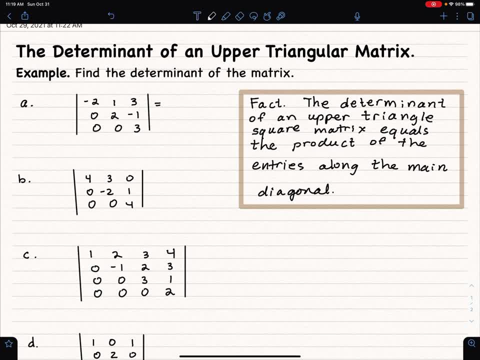 So I'll just go ahead and evaluate the determinant, which is a number, the determinant's a number, By multiplying those terms along the main diagonal. The maybe terms is not what I'm supposed to say. entries. So those guys there, and then it's up to me to make a mistake. 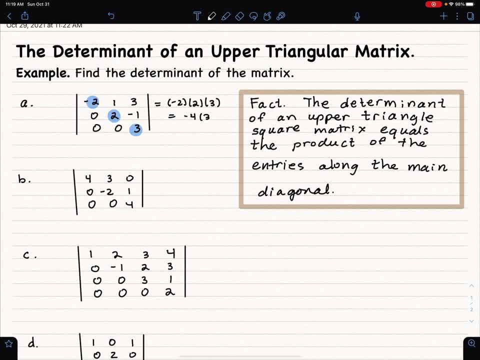 That's the negative. 2 times 2 is negative 4, multiplied by 3, and that's negative 12.. And hopefully that's correct. I mean, I think so. It's just the only question of whether I'm multiplying correctly. 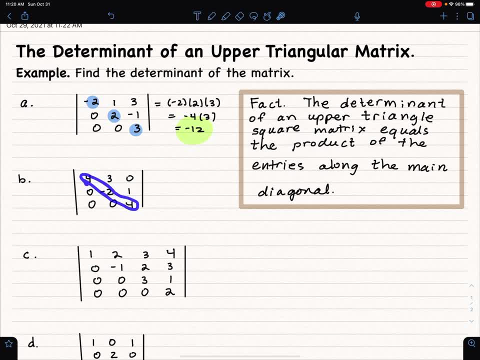 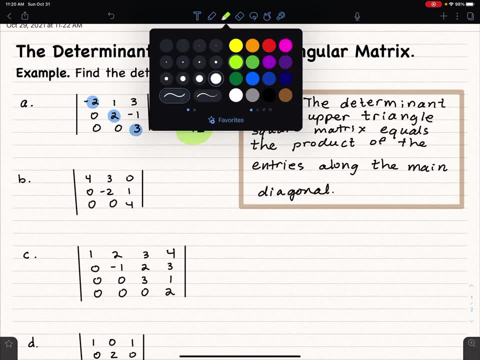 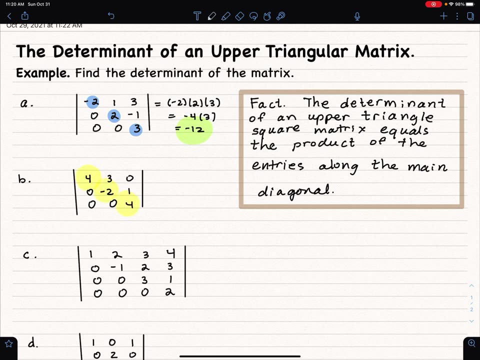 Okay, Here we go. We're going to multiply along the main diagonal because we have zeros below. By the way, the same statement is true for upper triangular matrix. Upper triangular matrices have zeros above the main diagonal. Alrighty, So here we go.